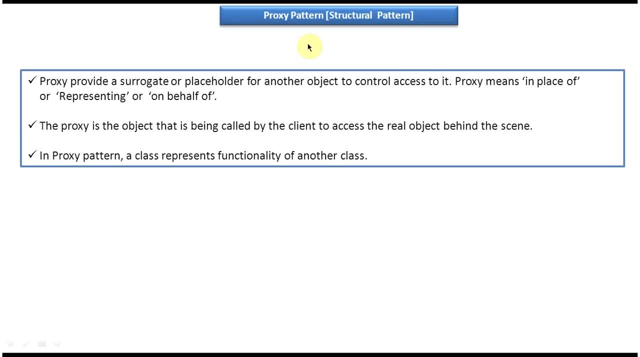 Hi, this video tutorial I will cover proxy design pattern introduction. This proxy pattern falls into the category of structural pattern. First we will see the explanation of proxy design pattern. This is the first explanation I will just read out. Proxy: provide a surrogate or placeholder for another object to control access to it. Proxy means in place of, or representing or on behalf of, And meaning of surrogate is act on behalf of others. So what is the main work of proxy? is it works on behalf of the real object or it represent real object? 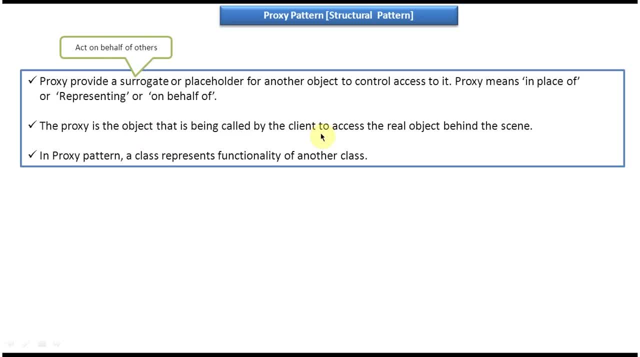 The second explanation is: proxy is the object that is being called by the client to access the real object behind the scene. And the third explanation is: in proxy pattern, a class represents functionality of another class. We will show you one diagram so that you will understand these explanations. 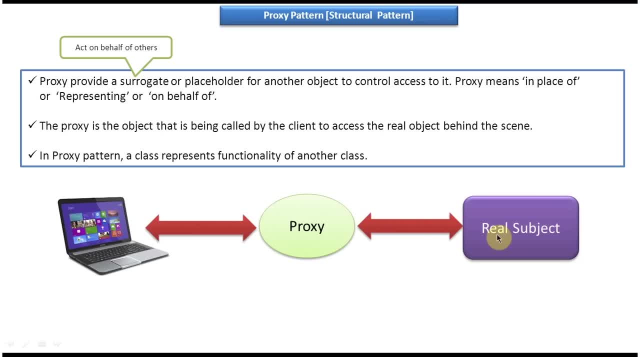 So left side you can see client, right side you can see real subject and center you can see proxy. So what is the main work of proxy design pattern? Suppose this client wants to communicate to real subject, then it should communicate via proxy, as per the proxy design pattern. 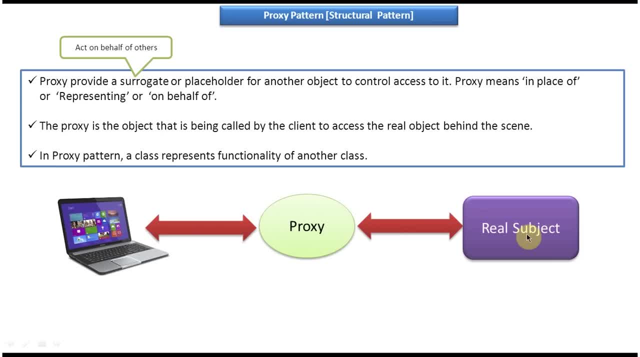 So if client wants to access some methods in real subject, then client will send request to the proxy, then proxy will make request to the real subject And there are four kinds of proxies are there. The first one is remote proxy. second one is virtual proxy. third one is protection. 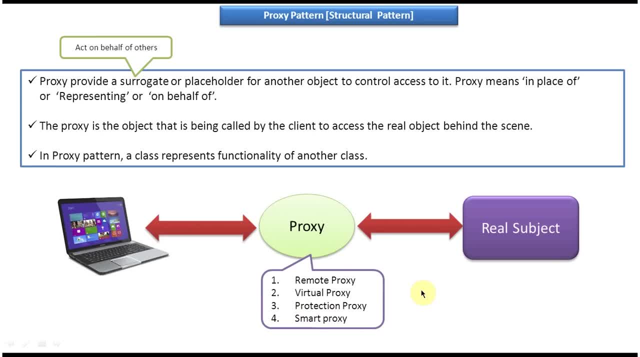 proxy. fourth one is smart proxy. And what is the need of proxy design pattern and when to use proxy design pattern, I have explained in the separate video tutorials. I have created Proxy design pattern real-time example video tutorial: proxy design pattern class diagram. 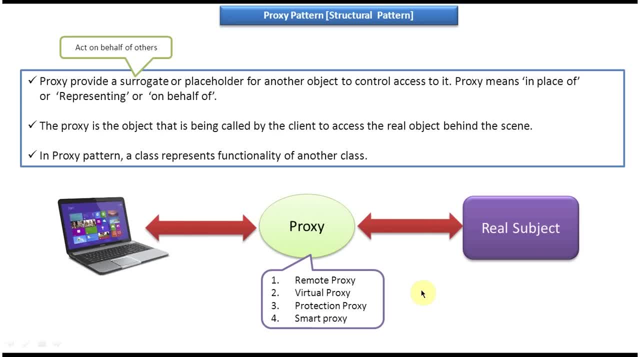 sequence diagram- video tutorial. and proxy design pattern implementation video tutorial. So if you want to know more about this proxy design pattern, please log into my channel and watch those videos. And this is about proxy design pattern introduction, and thanks for watching. bye.